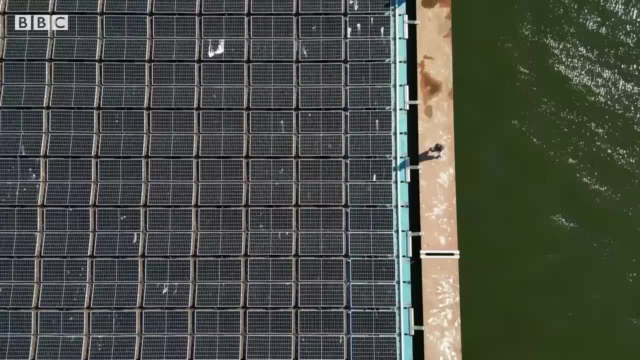 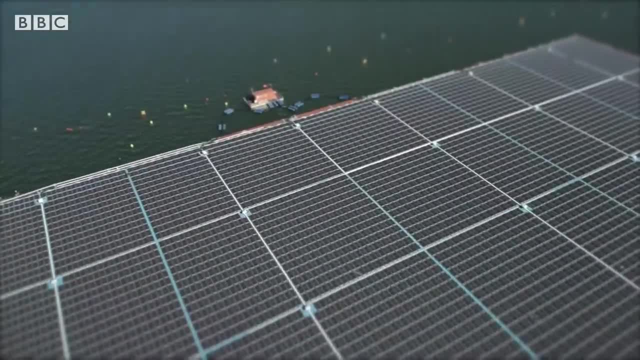 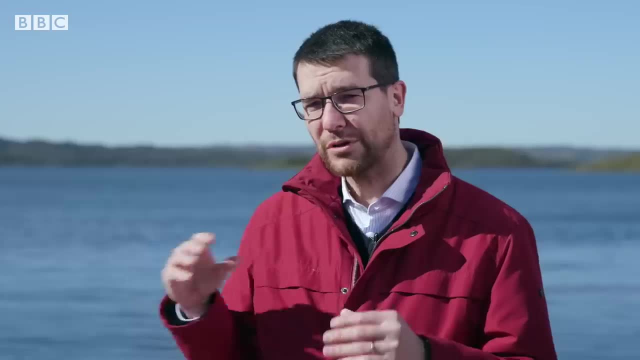 the solar farm will recoup its investment in a decade. But there's a particular reason why the solar farm was built at this spot, Namely its proximity to the Alcava Dam. The hydro-electrical plant only uses one-third of the capacity of the power line, So we have 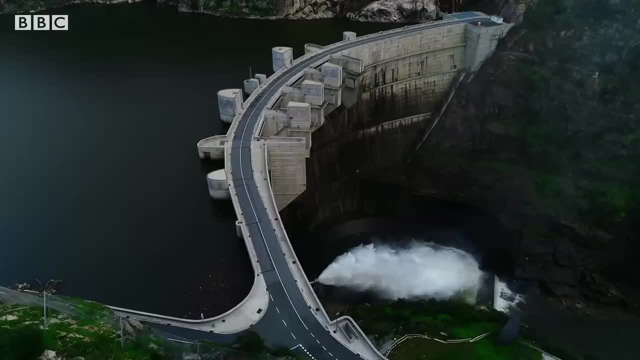 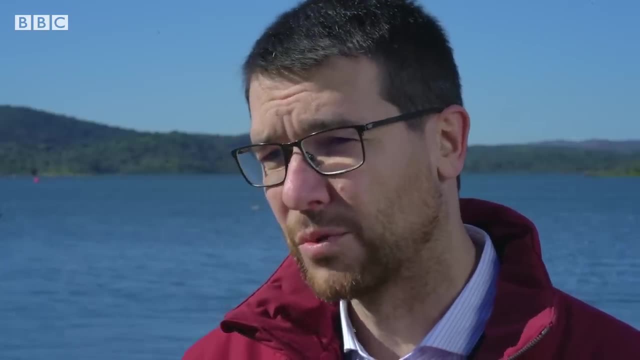 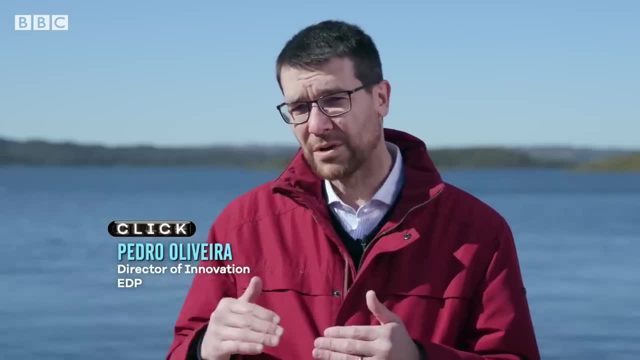 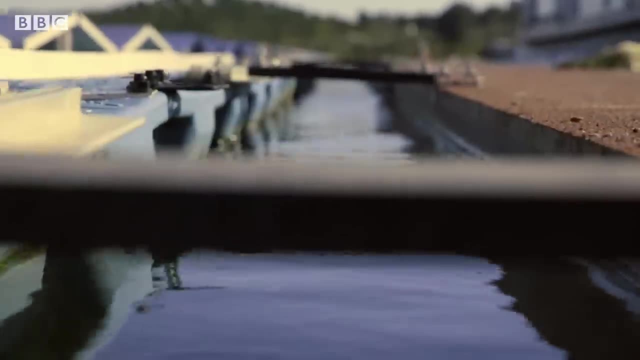 So we created this hybrid construction. This is just an example. So we created this hybrid construction. So we created this hybrid construction. So we combined solar and hydro power on the same power line, sharing the same infrastructure. But there are other benefits to having the solar platform on water. 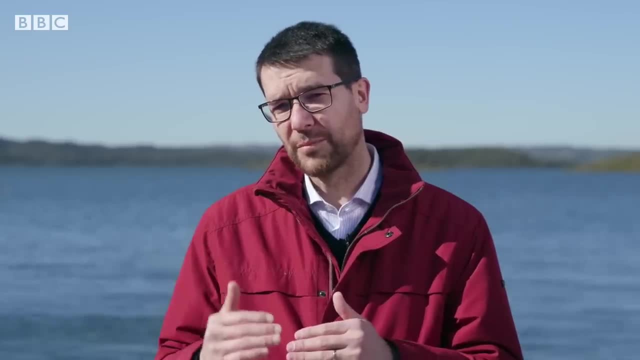 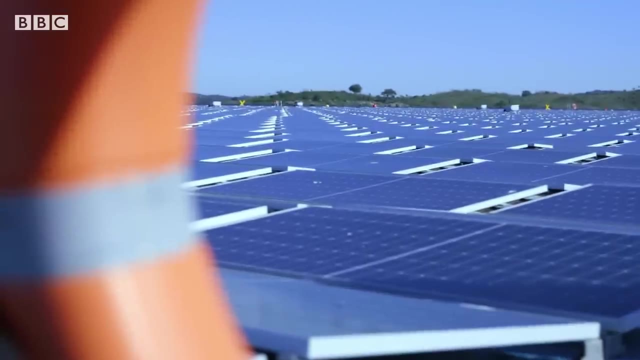 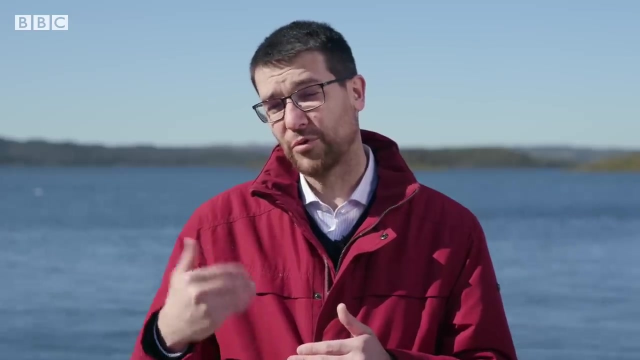 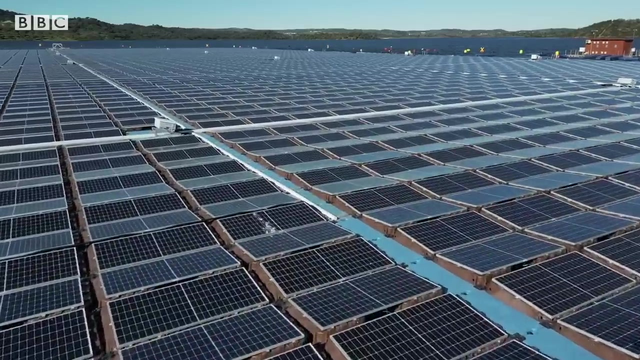 Being closer to the water surfaces. We reduced the temperature of the panel and then we increased the efficiency of the panels. We observed an increase in efficiency up to 10%. An annual average increase of around 4% increase of production. Large platforms like this one also cool water temperatures by shielding the surface from. 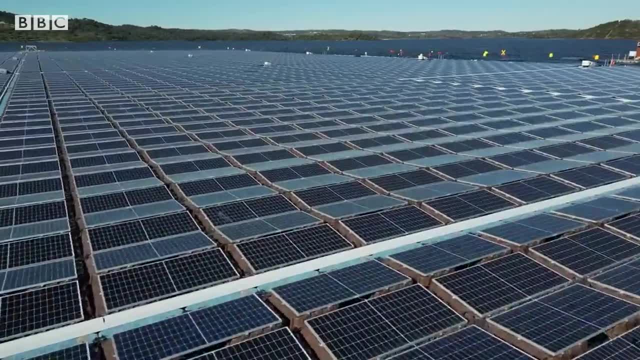 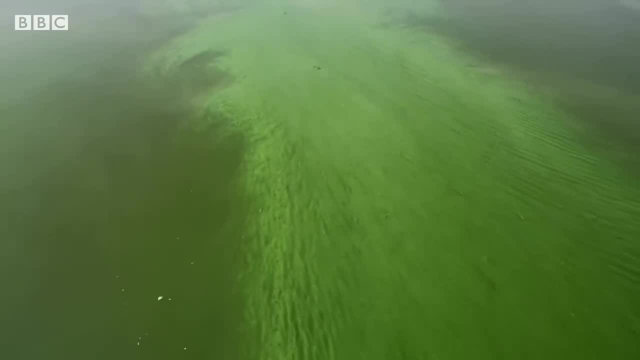 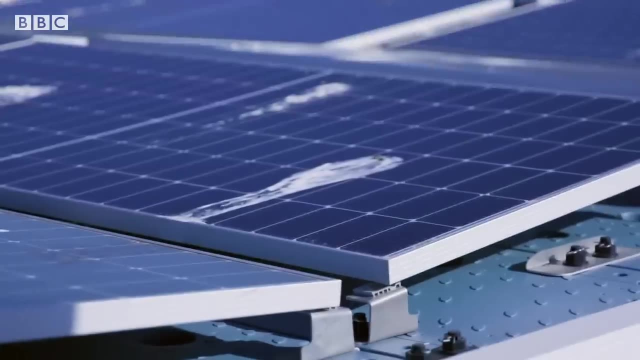 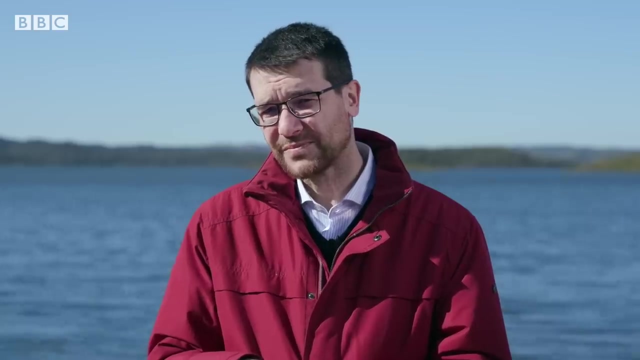 the sun. This not only reduces evaporation but prevents the growth of blooms of blue-green algae, which can produce harmful toxins. But there is one rather messy downside to having such a large platform on the water, And one thing that I couldn't help but notice when we were looking at the panels is the 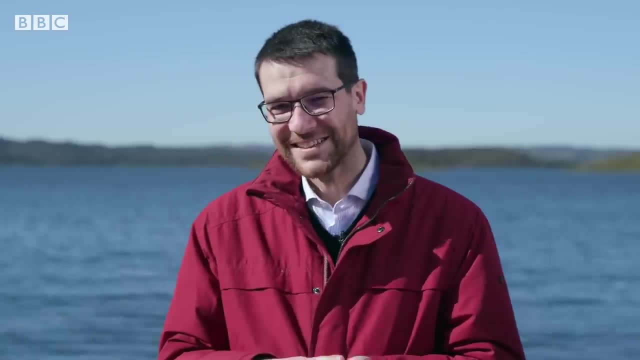 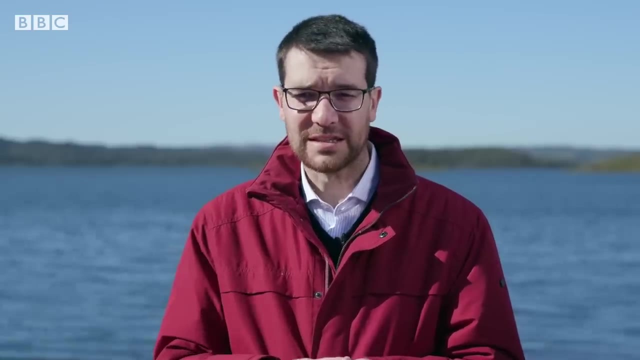 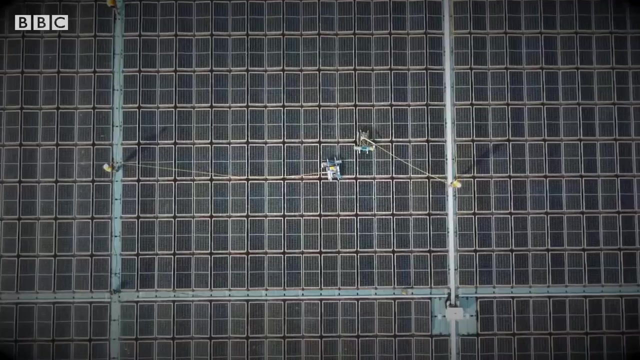 local birds leave some gifts behind. What kind of impact does that have and how do you manage that? When they are very dirty, it has an impact on the efficiency of the panels. We are doing some proof of concepts with the robot. We have the idea to have autonomous robots doing.